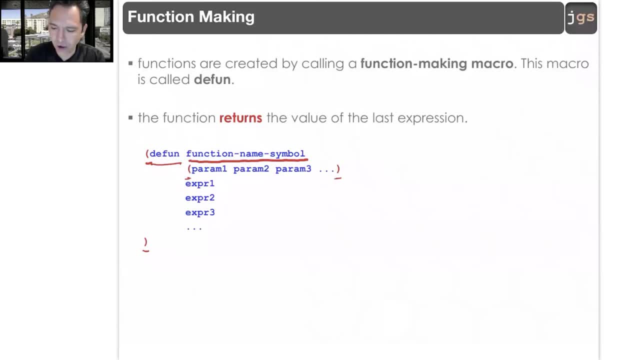 because you are creating a list. So all this is the parameter for the phone. The parameters do not have a type, So the only thing that you need to provide is the name for the parameter. So, in this case, one, two, three parameters, And you can put as many as you want. So you 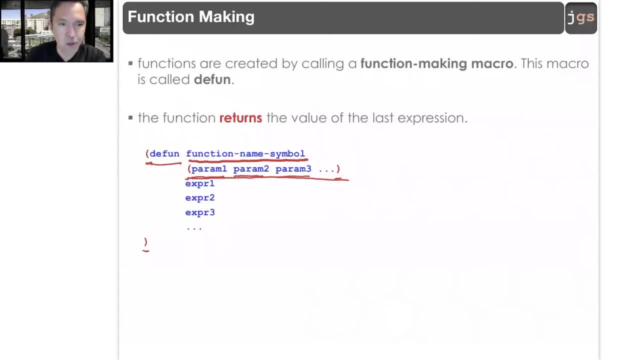 can put as many as you want. So you can put as many as you need. You put only the name, Do not need commas. The white space is the one to separate one parameter from the other. After that, the body of your 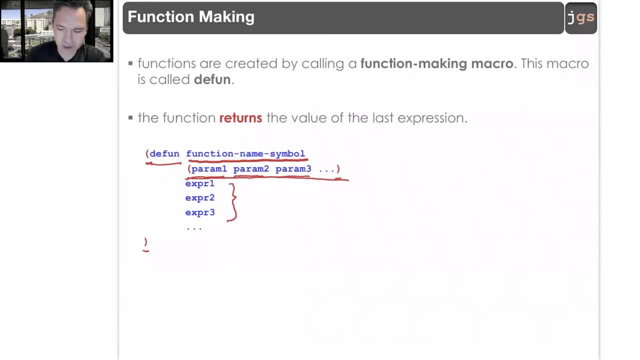 function, Whatever you want your function to do, And you close the definition, as we mentioned before, with the closing parentheses. This is what you need to do to create a new function. Now, any function is going to return something. And, as usual, your last line: 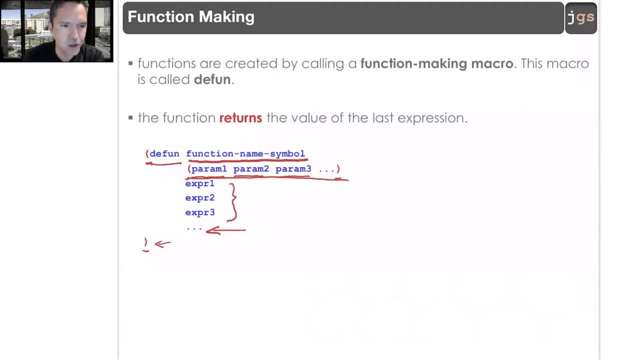 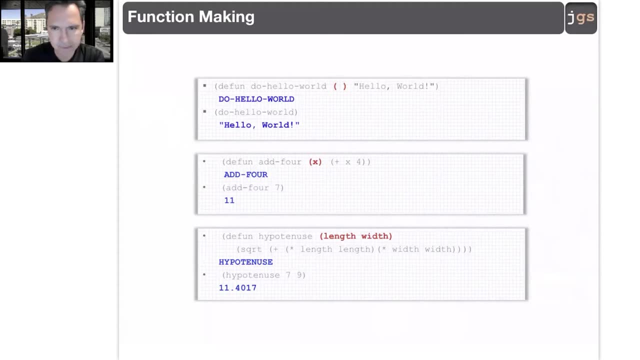 is going to define what your function is going to return. But I am going to show you some examples about it. Examples, Easy one: I want to create a function that is going to return hello world. So, Open parenthesis, Closing parenthesis Could be one line, Could be several lines. Remember: 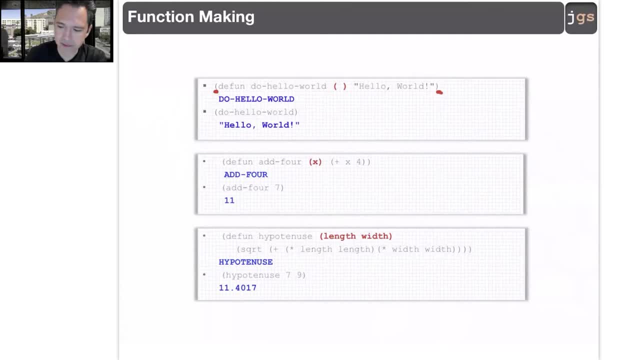 the enter is not relevant. Open parenthesis. Closing parenthesis. Definition of a function. The name for the function is doHelloWorld. I put several words together to play with this, But you can use only one word if you want, Even if the function does not receive. 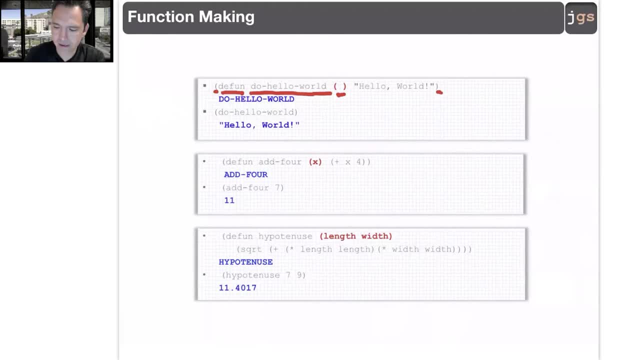 parameters. you need to provide A list as the second parameter of the definition of the function. So if you are creating a function that does not receive parameters, well, you can put here an empty list. So open parenthesis, Closing parenthesis. Nothing inside. Therefore the function does not have. 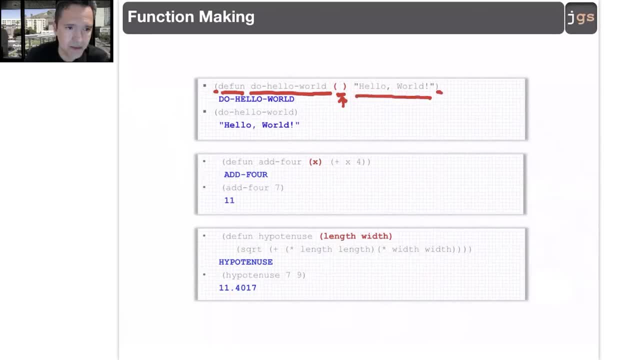 parameters, And then the instructions. The only instruction that I am adding here, helloWorld A string, Something that we mentioned before. If you put a variable or if you put, like in this case, a value, what is going to happen is that that is the value, that the function. 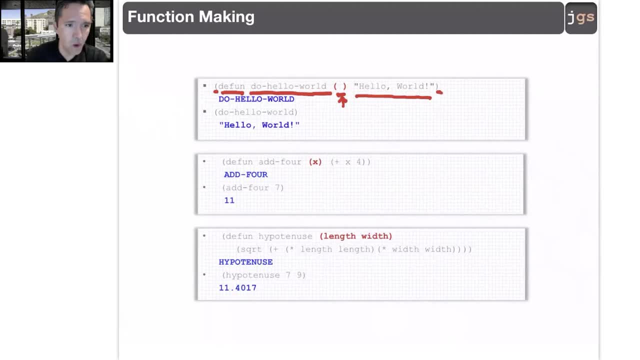 is going to return This example. what I am doing is doHelloWorld. Not parameters, but a string: Open parenthesis, Closing parenthesis, Nothing inside. Therefore, the function does not receive parameters. And then the instructions. The only instruction that I am adding here: helloWorld. 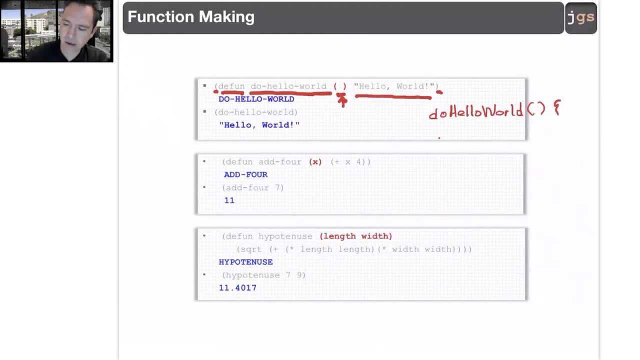 Not parameters, And the body is basically something like that. Now, lists do not have types, But if you want to do something like this, maybe what you want is…. Because I am returning hello world, I know that the return type of the function should be something. 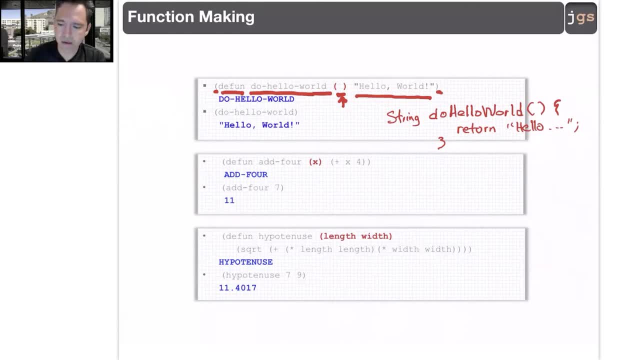 like string. So this could be the key element for that, And yeah, So let's finally pass theseین of the code that I am showing you here in Lisp Now in order to use your function. this is the function definition, and the function code is going to be: 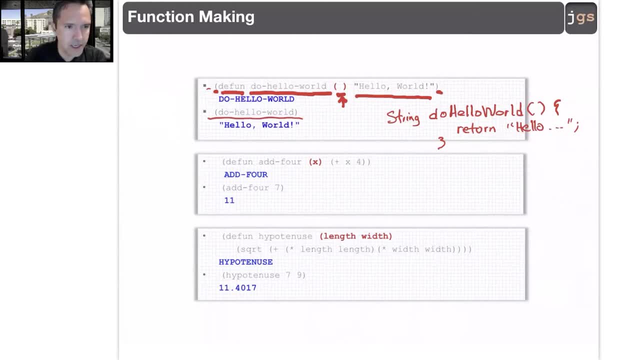 something like this: one Notice: I am calling a function. the syntactical rule is open parenthesis- ID of the function: parameters. in this case, we define that this one do not have parameters, so you close the parenthesis: DoHelloWorld. inside of parenthesis is the code for the function that I create with the. 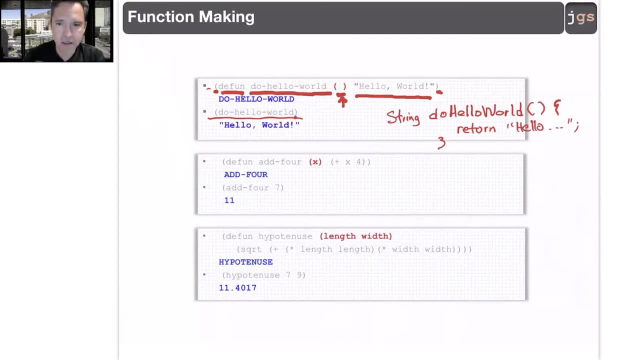 func- No parameters. You put nothing but the name of the function and you're going to have as an output immediately the value that you return. Now, This one is the output. when you call the function This one. what Lisp is going to show you after you create a new function is going to be: 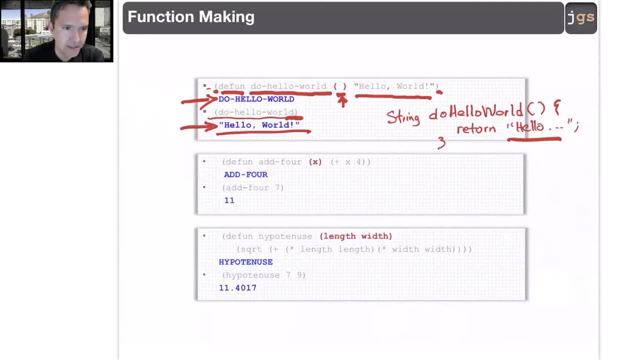 the name of the function that you create in uppercases. So whatever name you put to the function is the thing that is going to be printed here as a result. So basically the confirmation that Lisp gives you to tell you: hey, now I understand. 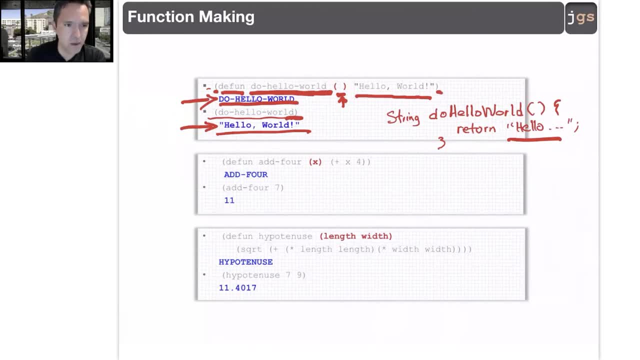 a new function and the name for that new function is this one, and it's going to give you that name in uppercase. Definition of the function. calling the function. Second example: open parenthesis, closing parenthesis. Instruction the full. I am going to define a new function. 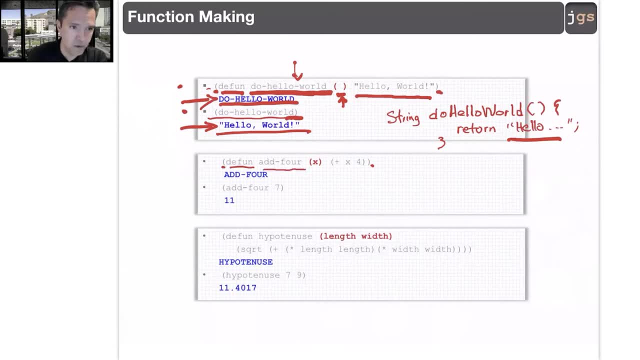 Name for the new function: Add function: Full. One ID Parameters: One parameter. And the name for the parameter x: Without data type, We do not use data types right. And the body for the function: The body: an addition. 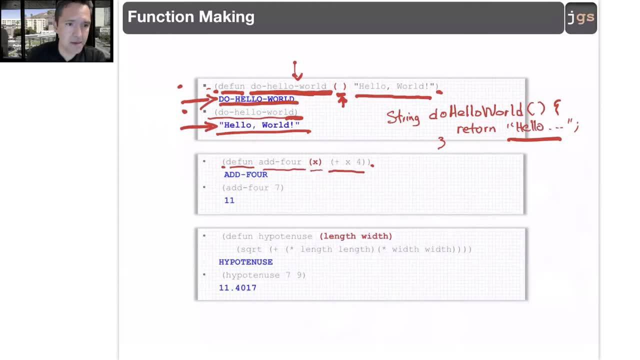 I am adding 4 to whatever I receive as a parameter, This one in Java. well, Name for the function: one parameter and the body. This one is the last line of the function, So that is the line that is going to be returned. 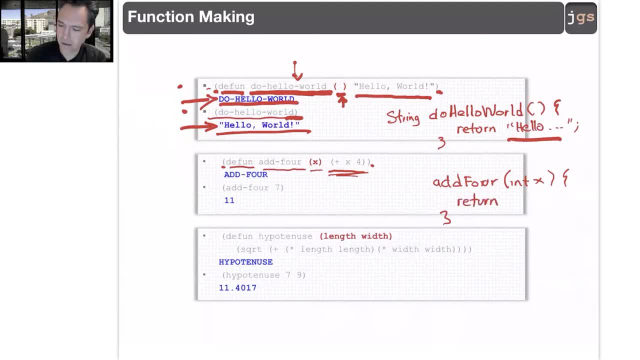 So a return x plus 4, and x is the variable that you receive as a parameter. So I receive a number and I return a number. So the type for this one could be integer. This could be something like the equivalent for this one. 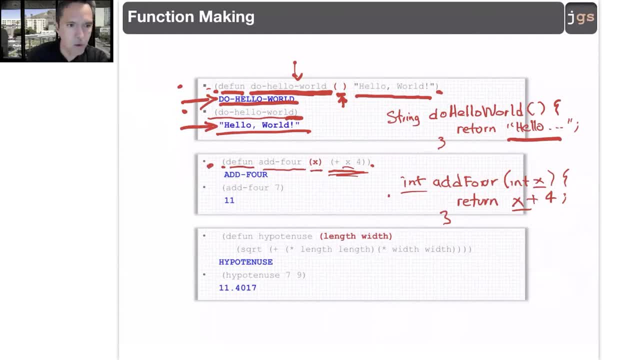 Now this is the definition When you want to call the function. open parenthesis, closing parenthesis. Now we use the name of the function as the one that we want to execute. We do not need the full And, in this case, one parameter. 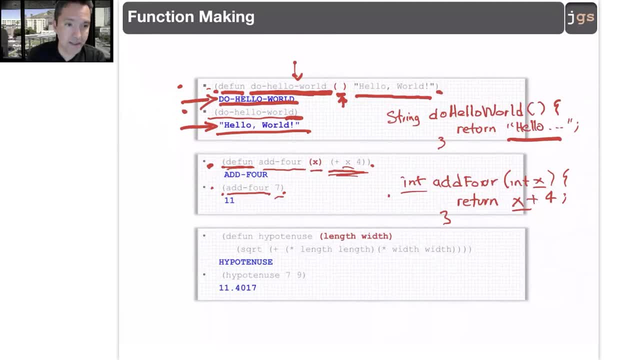 So I put as a parameter 7, and I am going to get as a result 7 plus 4.. And that result is the one that is going to be printed. So, without parameters, with one parameter, Without parameters returning a string. 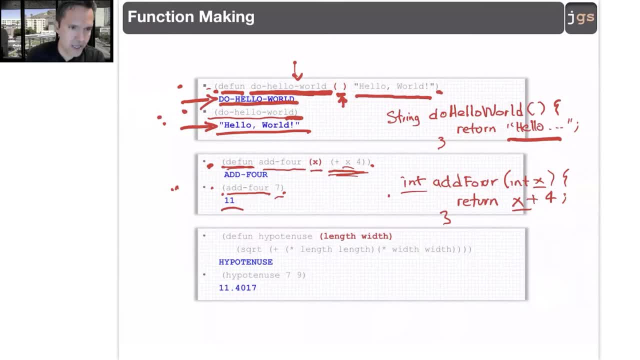 With parameters: receive an integer, return an integer- The last one. Definition of a function, Aim for the function And how many parameters. Two parameters: The first one, The second one And the return of this function. the body of the function is the next line. 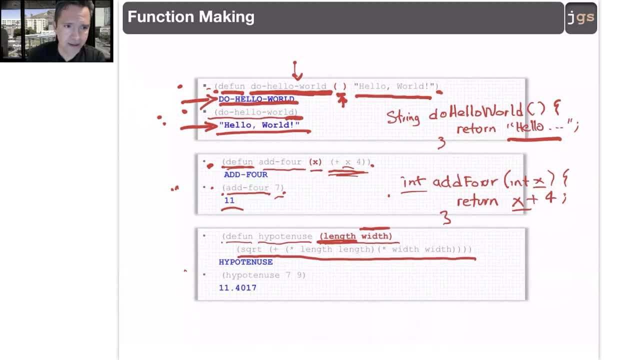 As I mentioned before, you don't care about the enters. They are not important. The only thing is, because this parenthesis is going to be closed here, everything inside is the definition of a new function. So for this function I have one big line. 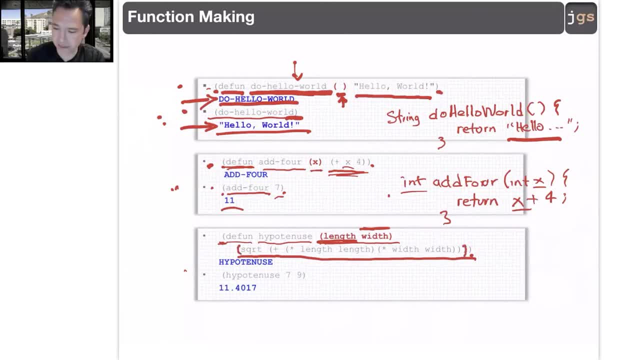 and the body is starting from the center. I am going to do a multiplication of the first parameter times the same parameter and the same for the other one, And then I am going to add the square root. So I am doing this calculation of the hypotenuse of a triangle. 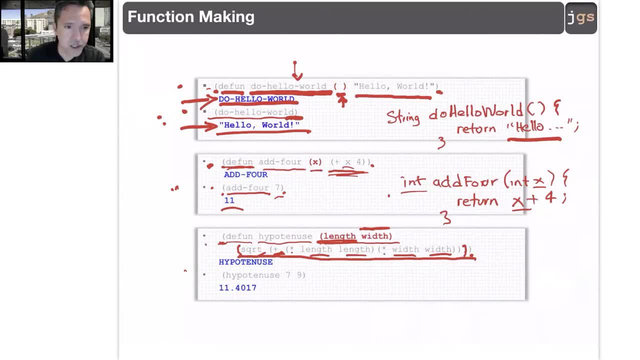 In this case, for this function. this is the definition And when I call the function, it is open parenthesis- closing parenthesis. name: the name that I provide to the function and the value that I want to use for the parameters. 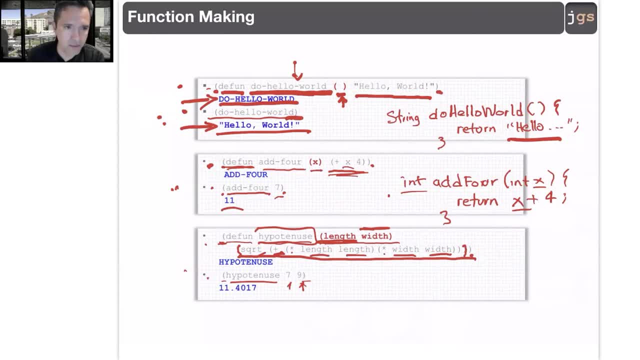 So in this case, I have a triangle, The measure of the size is seven and nine And I calculate the value for the hypotenuse And that is the value. That is the result. So no parameters, one parameter, two parameters. 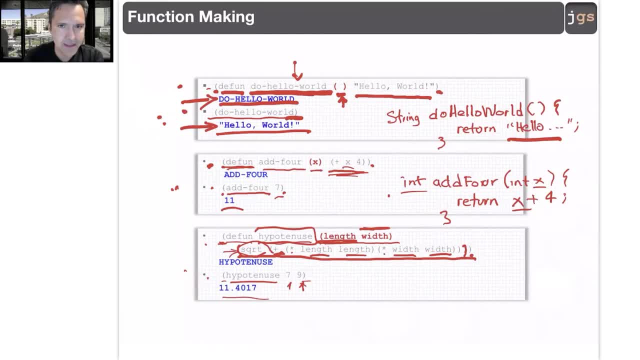 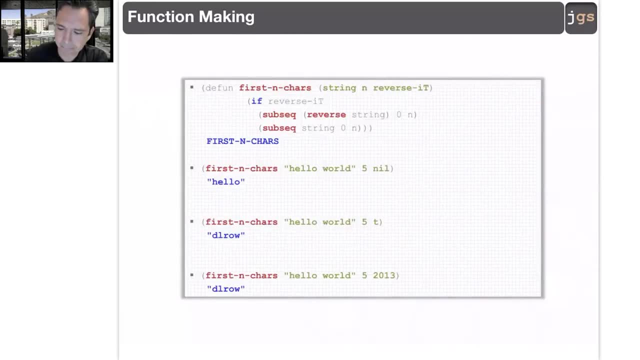 Hopefully you notice the model. That is the way that you create functions with Lisp. So more examples. Definition of a function Name for the function in red. How many parameters for this function? first, n charts: Good three. 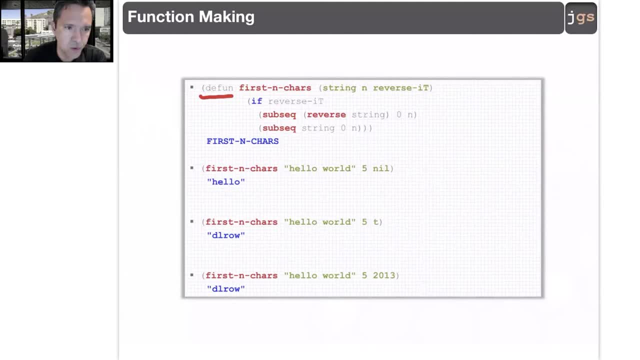 So notice that the only thing that you need to do is to check for the white spaces. Notice that even though I use string n and you can think like, oh, data type, string name n, just thinking about the previous languages, 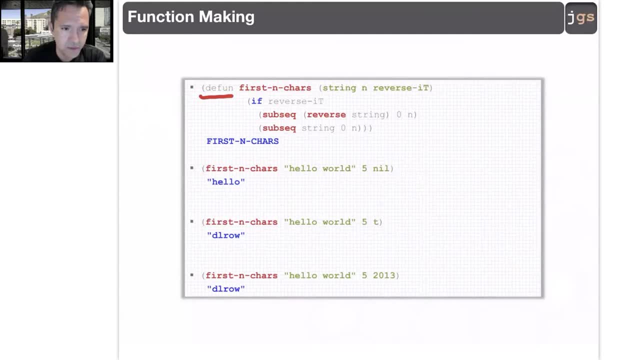 In this case, string is the name for the first parameter, n is the name of the second parameter, And notice that reverse it with the minus is one word. So that is the third parameter. So string one, n, the second and the last one, reverse it. 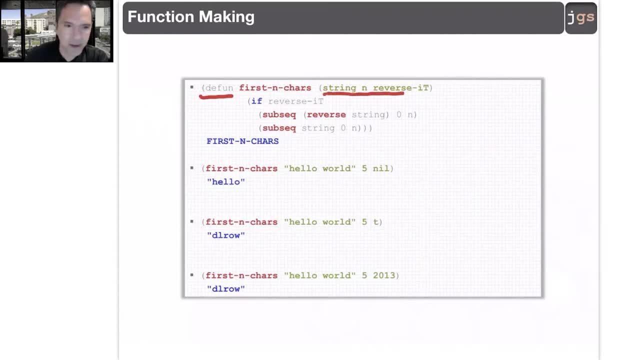 So my function with three parameters. Now I want to use if conditions. in the body of the function There is an if condition, So this is a method that have inside an if condition. Moreover, the condition, if you remember the if, is this one. 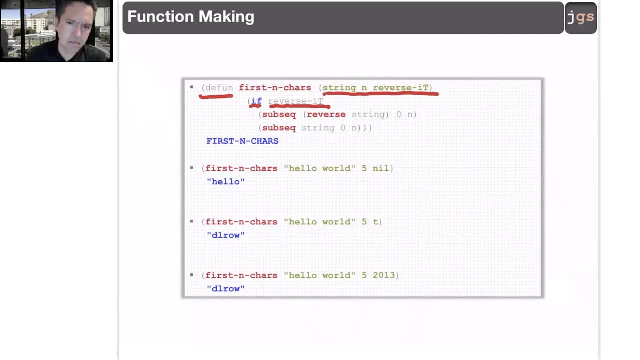 The condition is used one value. That value is going to be true or false, Well, t or nil. With that condition, this line is going to be executed if the condition is true. This line is going to be executed if the condition is false. 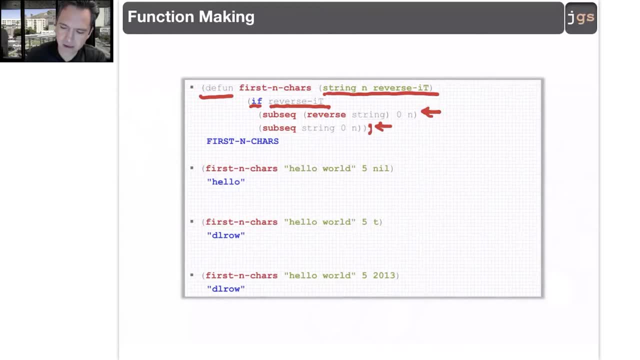 And I close the if here. So I have inside of my function, inside of my function, one if and depending of the if, true or false, something is going to happen. That something is the instruction subseq that we reviewed in the previous lecture. 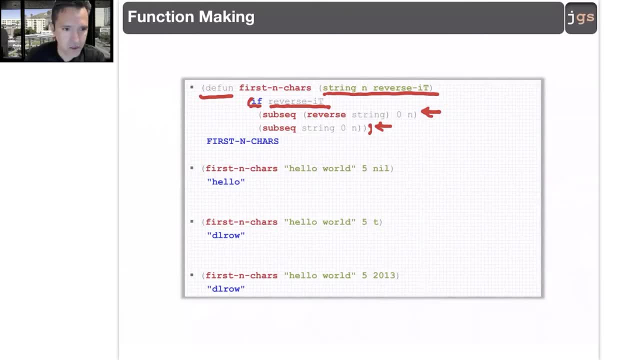 And if this subseq is executed, whatever is the result of that subseq is going to be the result of the if, But because the if is the last line, in fact is the only line, that is going to be also the result for the function that I am creating. 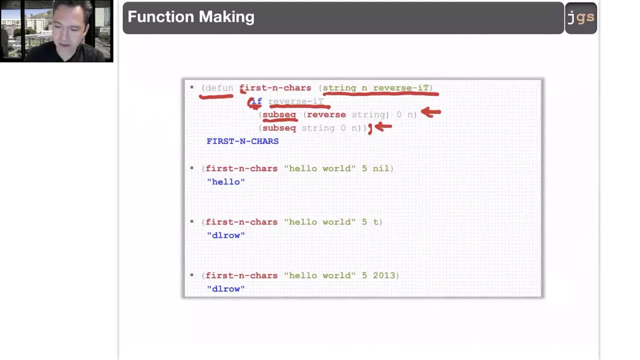 So basically I am returning the value that this subseq function returns, or this one if you are running the else part of the if So the same function, but in Java CC++ again we will have something like the return type could be a string. 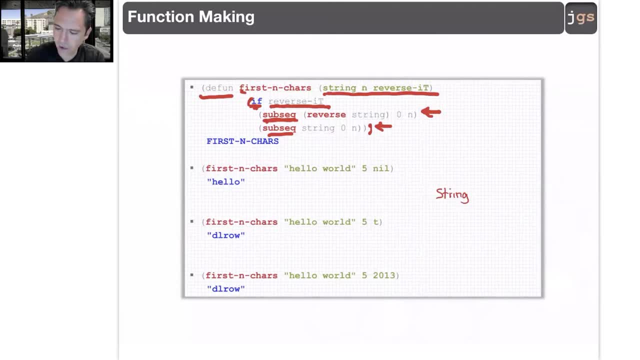 just because subseq is returning that We will have this name first and chart. You are using this upper-lowercase approach. We will have parameters and here we can think, like maybe the first one, even though it is called a string. 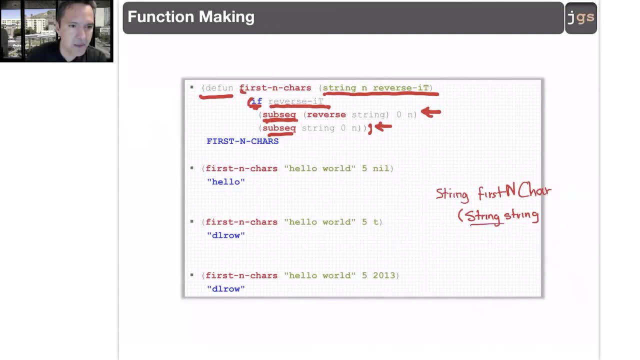 in Java CC++ you need a type. That type is going to be string, also with the s uppercase. the class We have n- n probably- is a number, so we need an integer number And we have this reverse it. 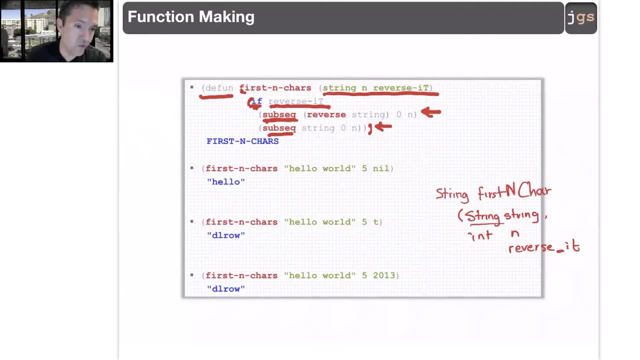 We can use the underscore, or if we follow Java, I can just make the i uppercase, So you decide. But because I am using that one in an if well, that one probably is a volume value, So this is kind of the parameters for my function. 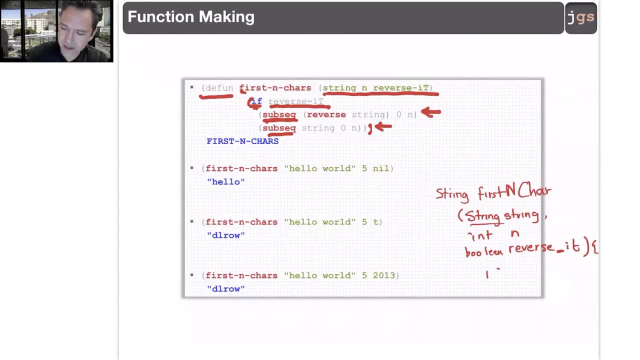 If I review the body, what I have in the body is this: if condition, the if condition is using as a condition the reverse it variable and that's it. I mean I am not comparing that one with anything, I just know that that one is volume. 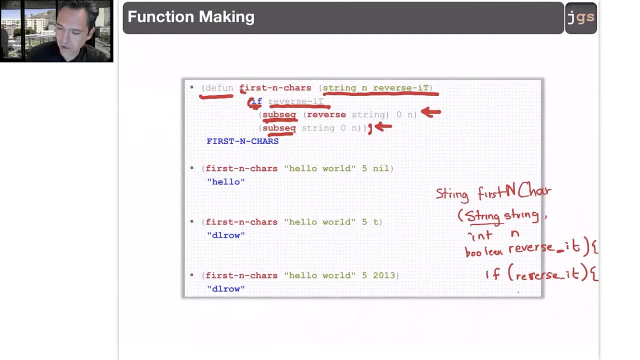 so it's going to be true or false and, depending on the value, I am going to return something here and I have an else part and in the else part I define to return something here. I close and I close. 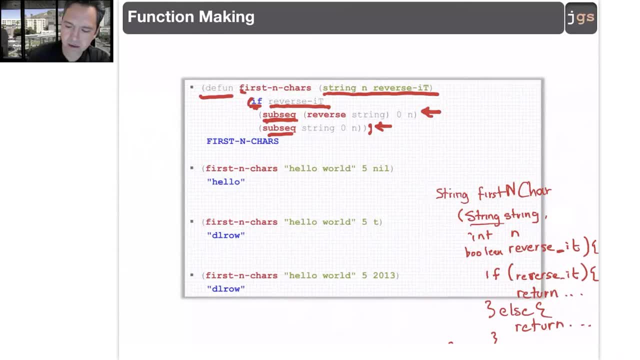 Something like that will be this one in the other languages. Now I can call my function and I can pass. the first parameter is hello world, the string, the second parameter is five and if I want to pass, the volume parameter. 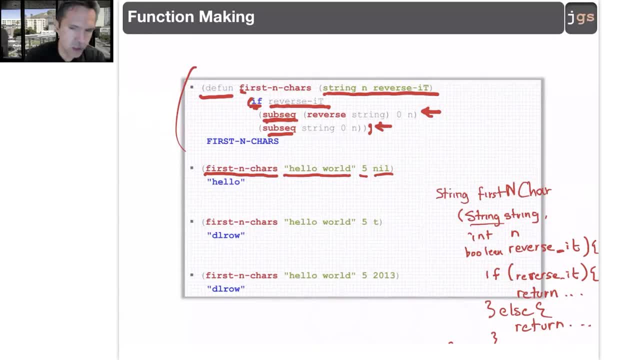 in this case, I can use nil false. therefore it's going to run this line, not the other one, and the resolution, which is hello, or I can use true as a parameter, and with the same input and the same number five. 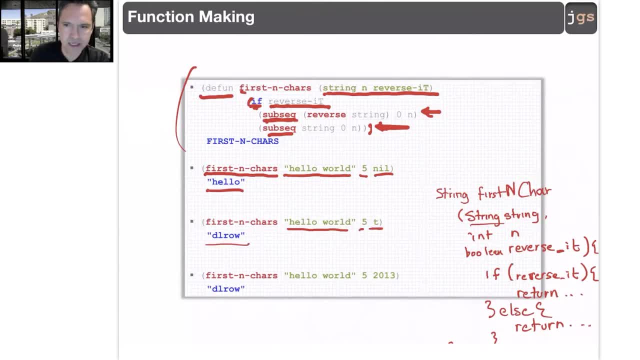 this could be the output, So you notice the subseq. the first one is using inside reverse, so you're going to return a subseq with the reverse of the string, and the other one is returning a subseq from the original string. 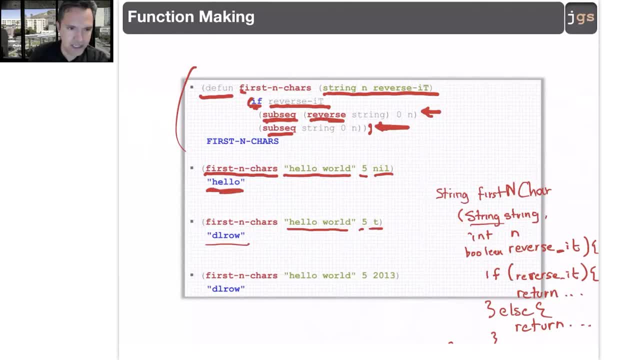 so the original one is hello, a subseq in the original one, starting in five: hello, the first five characters. in the second one I do the reverse, so this d becomes the first element, and so on, and I return the first five. 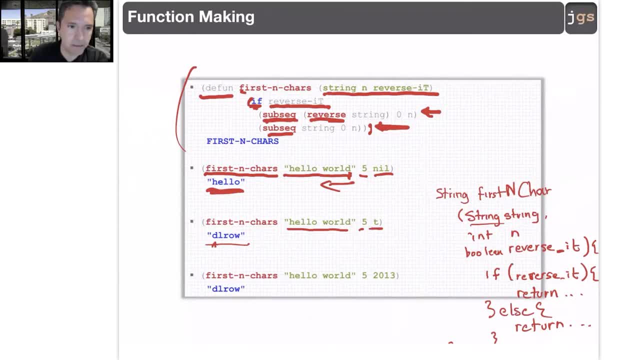 that become the last five because I applied the reverse. So, true or false, nil or t. One thing that you're going to notice what happened if, by any chance, I use as a third parameter something that is not nil. 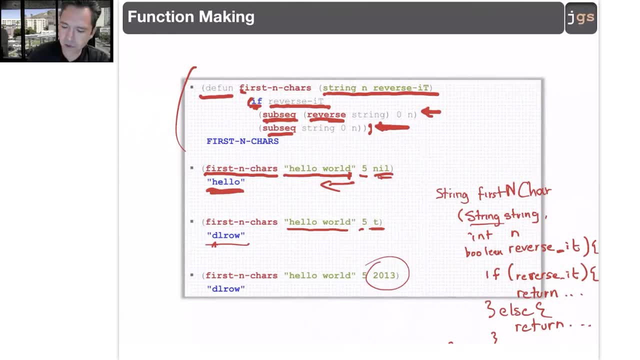 not t like I call my function. everything is the same as before, but here, instead of using nil or t, I put whatever a number. You notice the result. whatever you use, that is not nil. well, it's like. 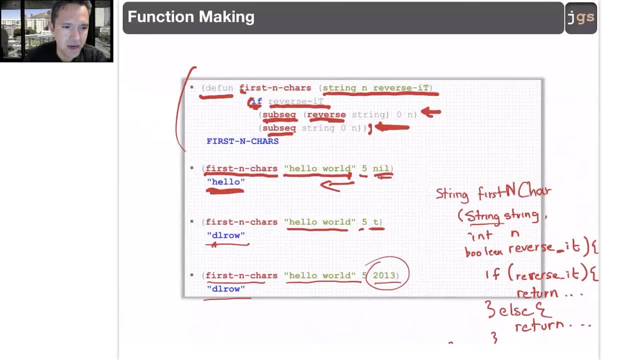 if you are not giving me false, then the assumption is you want this to be true. CC++- zero is false. whatever else you use, one or other number is going to be true. If you use nil, you want false. 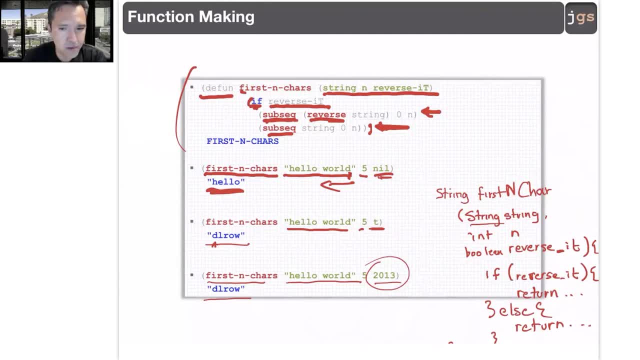 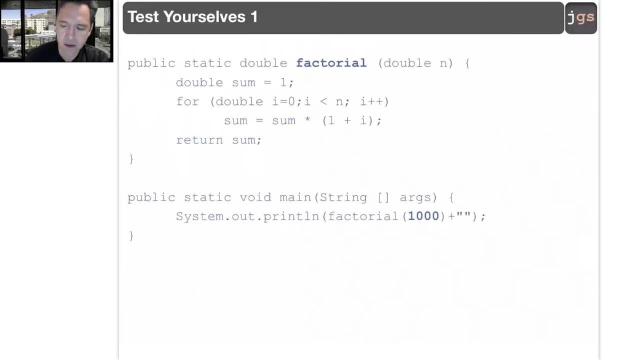 if you use t, you want true, and if you use any other thing but not, nil is going to behave like true. So I am sure that you remember this example. I am sure that you're familiar with the factorial function. 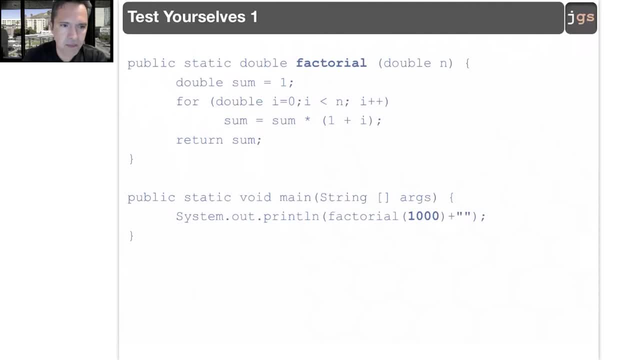 and I am sure that you programmed this one, maybe in the previous semester. this is java source code calling the function, defining the function right. So this source code is something that we can compile, run and we know what is going to be. 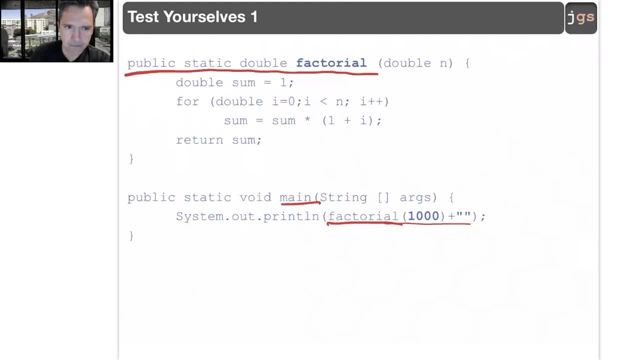 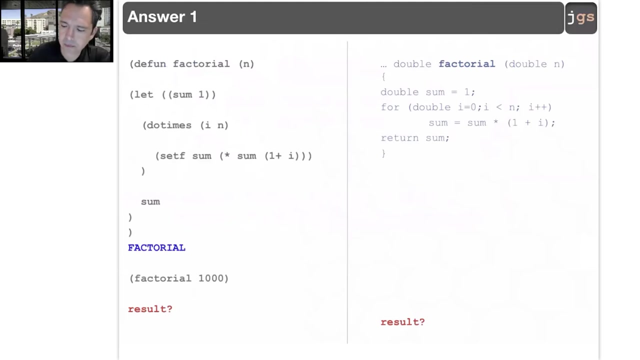 kind of the expected result. So what if I ask you to translate this from java to lisp? I am asking you for two things: definition of a function and call the function. And I put this column here with: 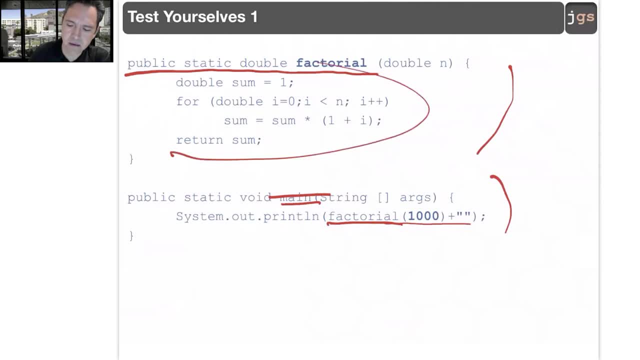 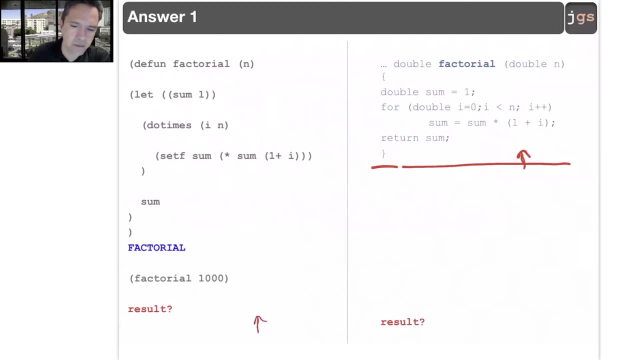 the same thing that you have before is basically this information: is this information used as a reference? What if I told you that this is the angle? So can we understand how we create this one from this one? 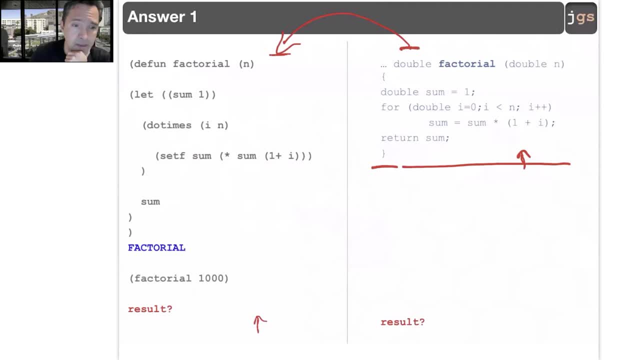 Let's see. The first thing that I have is all the modifiers from java. We can ignore those. The second thing that I have is this function is going to return double. I don't care about the type, the only thing that I need to remember. 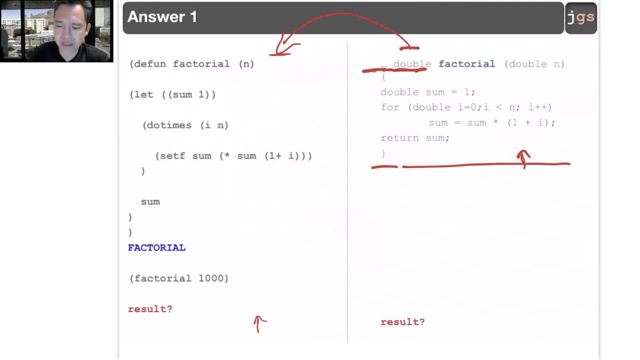 is that I want to return a number, But the type itself, I can ignore it. The name: the name is important, So I can start with lisp, open parentheses. definition of a function and I want to use a name for the function. 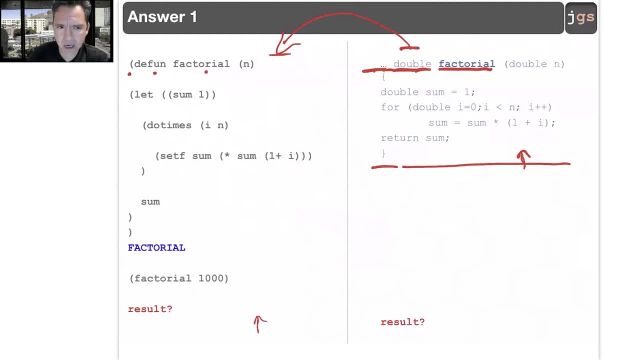 factorial. Then I have one parameter and I know that that one parameter is going to be a number. I don't care about the type. the only thing that I care is the name of the parameter. is going to be n. 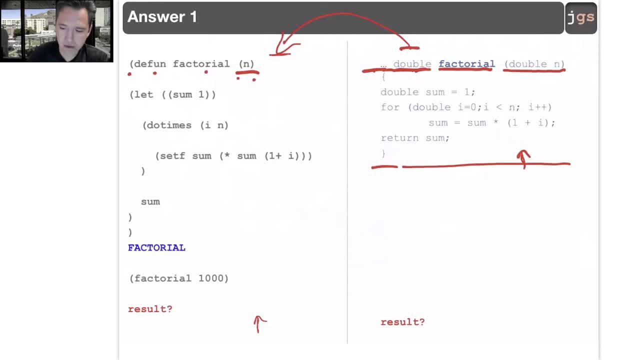 I need the parentheses because all the parameters should be together in one list And that list should be the second argument, the second parameter for the def function. So open parentheses, closing parentheses, and I want this one. 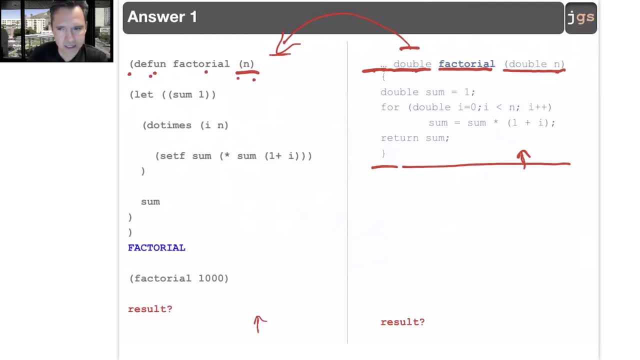 the parameter n inside. Next, Something that I read here is that I am doing a local variable and that local variable sum is equal to one. So we need a local variable. We want a local variable. 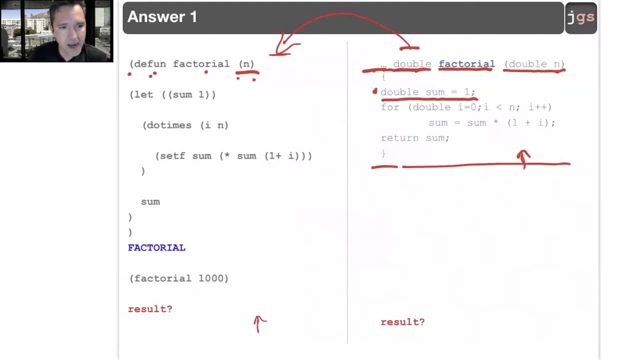 If you remember to create a local variable in lisp, we use let. So the first line for my definition of function, the first line in the body of the function factorial, is going to be open parentheses. 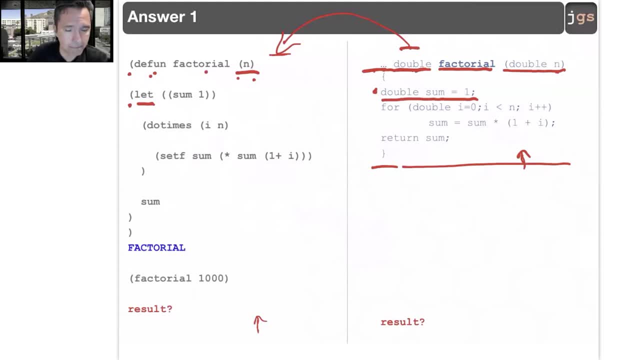 let, Because I want a local variable. Then the local variable that I want is sum And, in particular, I want that sum to have the initial value one. If you review, let the instruction, let receive. 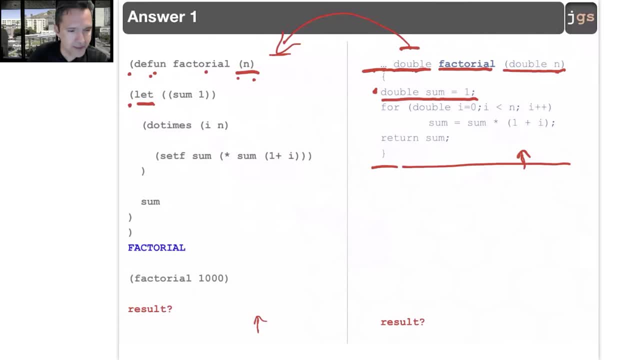 one parameter, the first one, that is, a list- open and closing parentheses, and that list have inside list a list of a list, of a list, list of elements, Which each element. 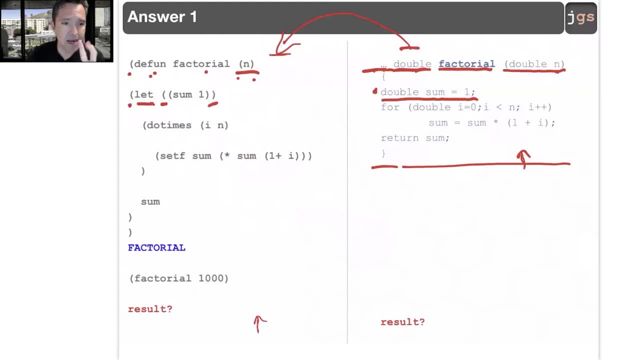 inside of the list is two things: The name that I want for the variable and the initial value for the variable. In this case, the list have one element inside another list, that is the name of the variable. 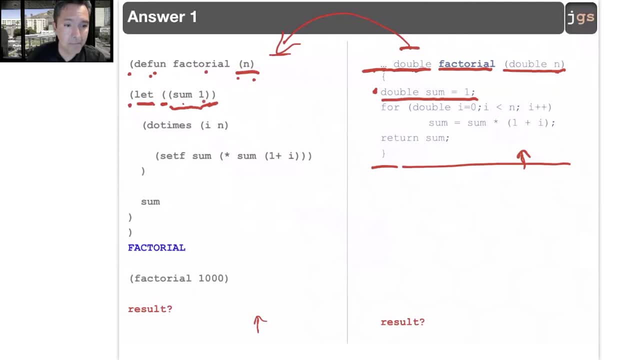 sum and the initial value. one Very, very important- two times open and closing parentheses. First, to enclose all the local variables that I want Inside, for each local variable that I want. 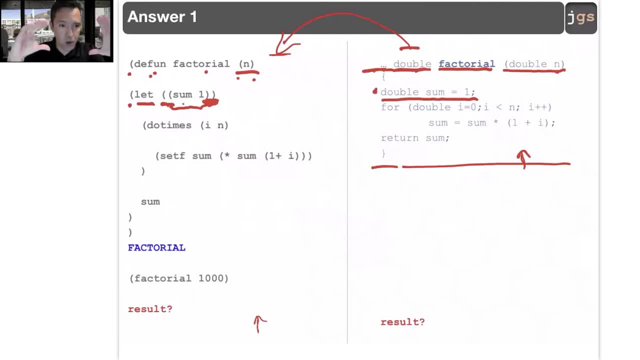 open and close parentheses because I am enclosing the name and the initial value. In this case, because I have only one local variable, is going to look like twice the open and twice the closing parentheses. 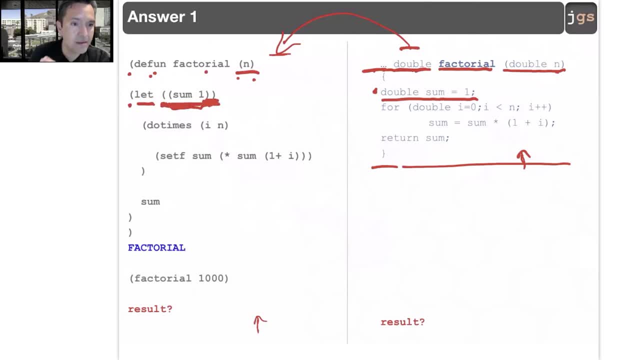 Now, after I define my variables, this, this open parentheses- is not going to close until the end, Because all the instructions that I want to use that local variable should be inside of the let. 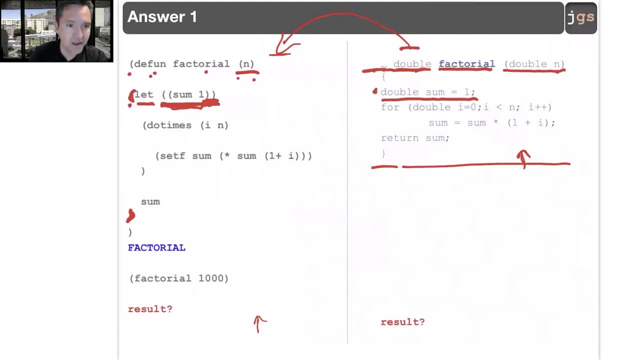 function Right. So open the definition of the function, closing the definition of the function. Open, let, closing, let. The body for the function is just one big let function And that let. 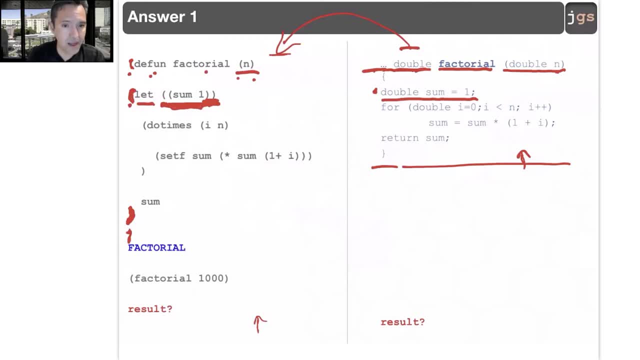 function have this local variable and then some lines, these lines that are going to be using that local variable. But well, let's review. Next line is a for loop And I want a for loop. 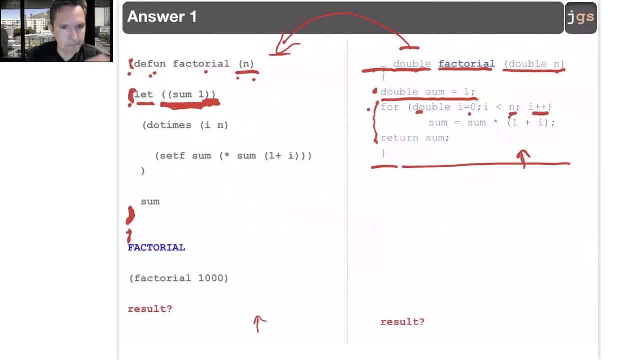 to go from zero to n, If you apply what we reviewed before here in Lisp, the replacement for that is our do times function. Moreover, for the do time you have, 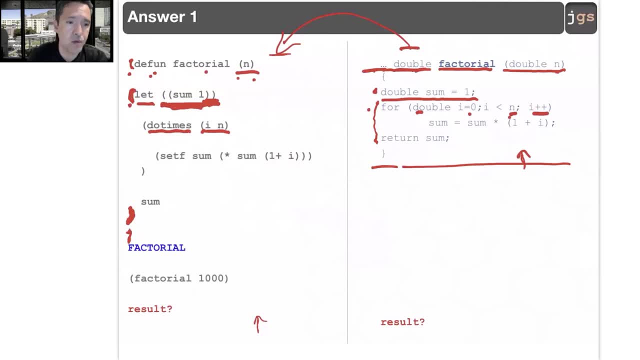 two or three parameters. In this case, we're using two. We are not specifying a particular return thing, And the only thing that we define is the name of the variable that I want to use. 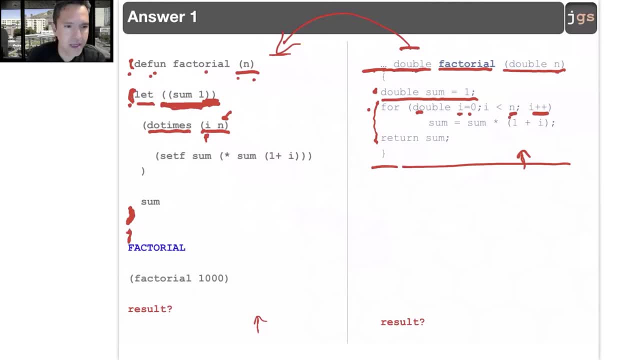 as a control variable for the loop I use. I here I am going to use the same used to do the equivalence, And the second parameter is how many times I want this loop to run And 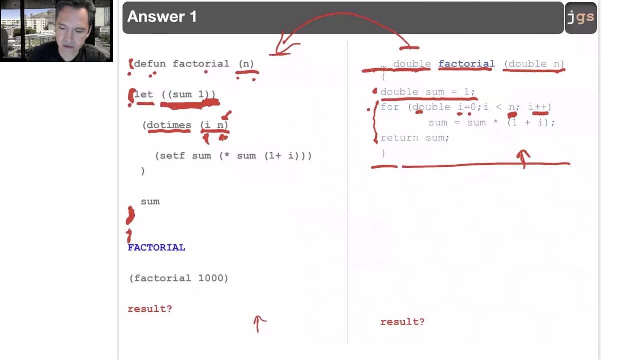 use like before. I want the loop to run n times, So name of the variable for the control how many times the loop is going to run. This one is equivalent to the for that I have here. 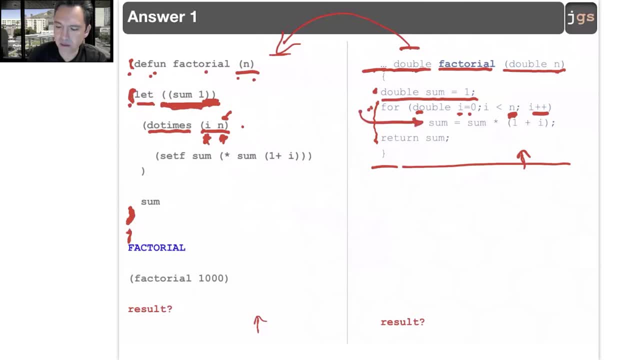 Now, inside of the, for what I want to do is this: sum equal, sum plus i. If you remember the replacement for the equal, the assignation is this: set f function, And that is going to be the. 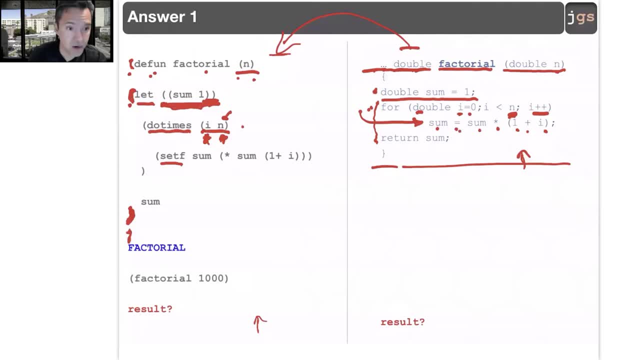 first one, just because the precedence of the equal, remember, is the last thing to happen. So the last thing to happen Then what I want to do is to do an assignation, set f. 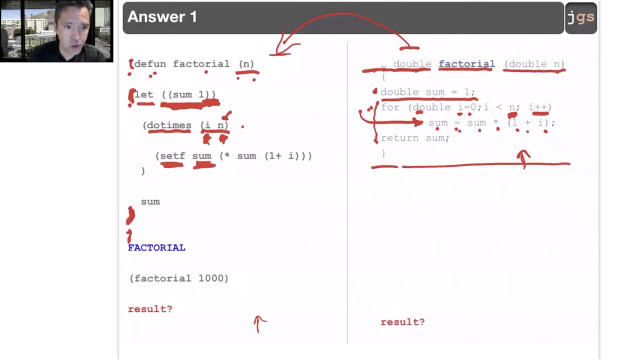 In sum, that is, to the variable that I'm going to use, and this is the operation that I want to happen. If you notice, first thing to happen, one plus i, You can do. 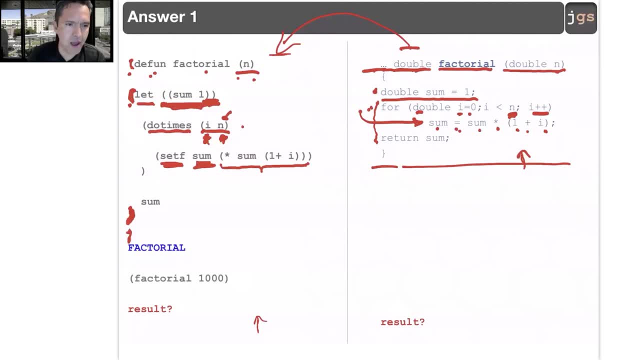 parentheses- plus i one, just to play with something different. I am using this one plus, remember the function that the incrementing one, and I am using only one parameter, i, But you can use. 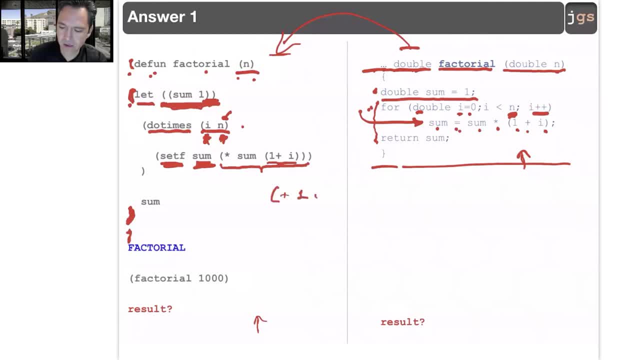 the plus, and you can use the one and you can use i. That is exactly the same. You can use whatever you prefer, So that the one is going to happen first And then a multiplication. 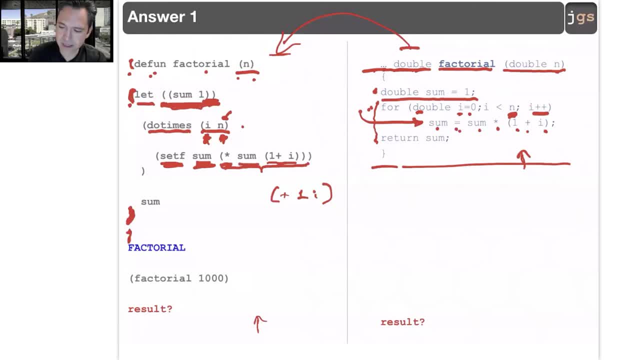 of that thing: times sum use, like is happening here, And then the set f. The last thing that I want to happen in this version is this line: return: sum, Now return. 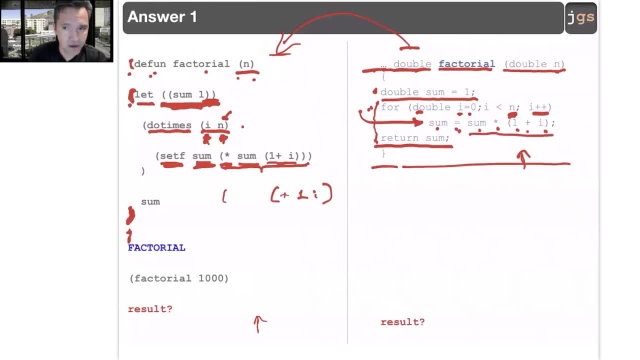 sum. in Lisp we do not have a return keyword. The only thing that we need to do is to put sum as the last line, in this case in the let instruction. Why? Because 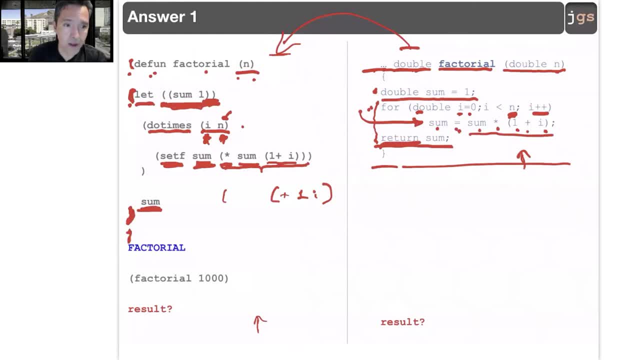 the let instruction return. whatever you put as the last line, Notice that we do not use the parentheses for sum, because sum is not a function, It's a variable, But that you put the name of the variable. 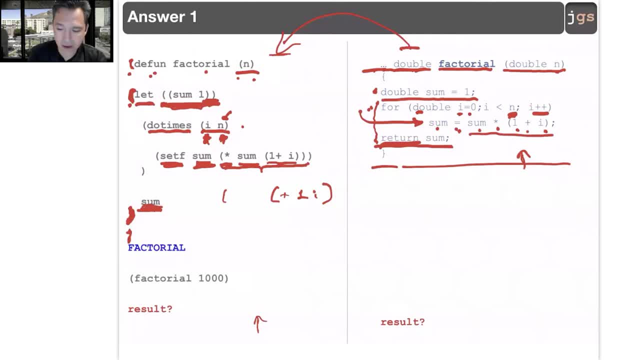 alone that one is going to be replaced for the value, And because this line is the last one, that is the value that let is going to return. Moreover, because let is the last instruction in the function, 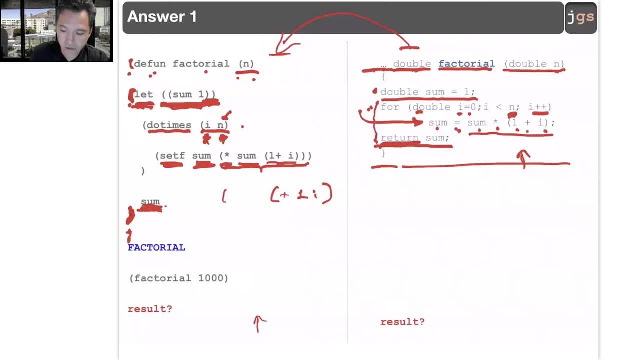 that is the value that also the function is going to return. So here is the definition list. is going to print the name of the function in uppercase, just to let me know that. now I understand. 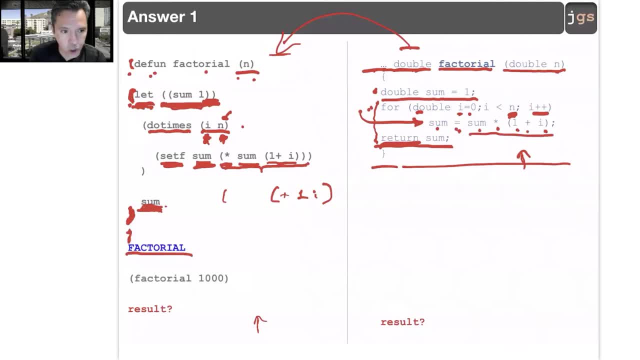 a new function. Now I learn something. Then I can call the function- open and close- parentheses- the name of my function- with one parameter. You call this one and here you have the result. Now I ask you: 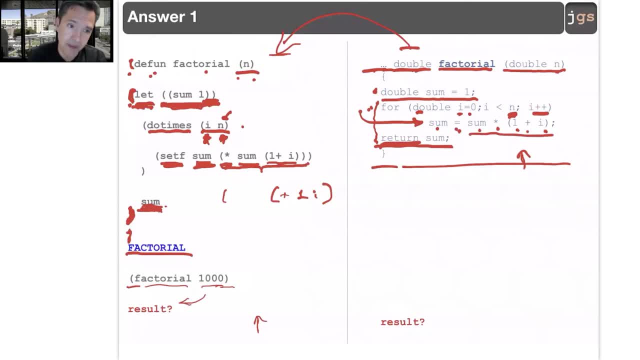 for the result, to call this one. and here you have the result. Now I ask you for the result, using the java version and the list version. Can you call this one the java version? 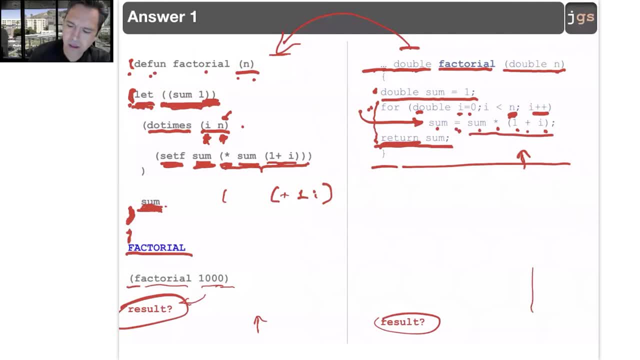 of the factorial method and ask for the factorial of 1000. And it's too big, So I'm going to call this one. and here, I'm going to call this one. 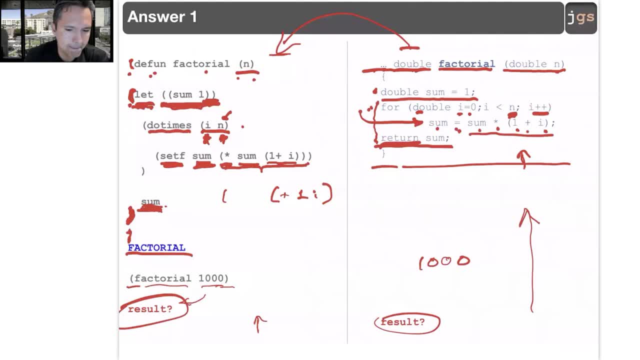 and here this one, and here this one, and here what is going to happen If you define the key valence in list and you use wrong this factorial of 1000.. You are going to. 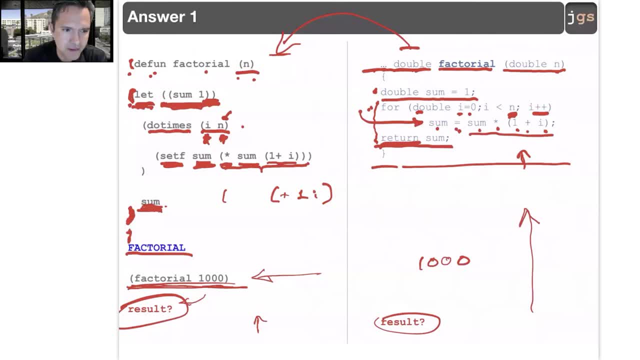 get the result. My advice: try, try both. I am sure that you should have this one in your computer. I am sure some time Try, Do this one, And I am asking the 1000, but you can try with other numbers. 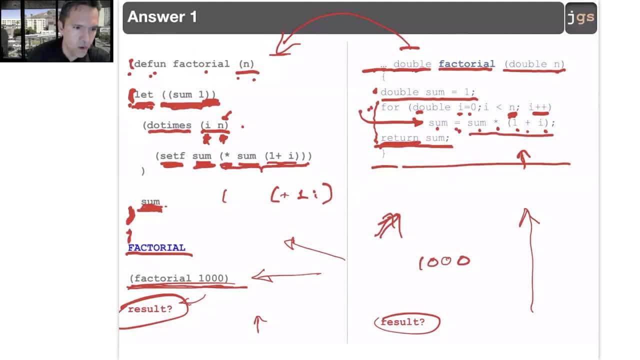 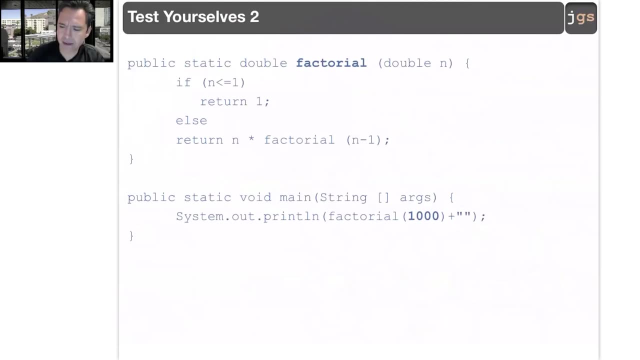 And you can notice what is the big difference between one and the other. And in the case of Java and Lisp, both are running with an interpreter. Now, I am sure that you remember this one. It's the recursive one, It's the one that have only an if-else condition, no loop, and 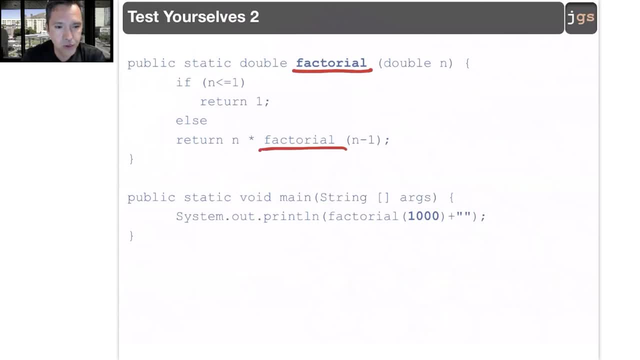 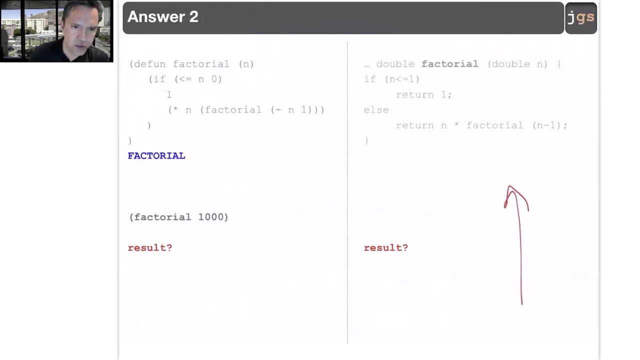 you calculate the factorial using a code to the same function: factorial. This is a source code, again with Java CC++, The equivalent in Lisp. This is the same that I showed you before, Just as a reference. I put the important elements in one column And this could be the equivalent with Lisp. 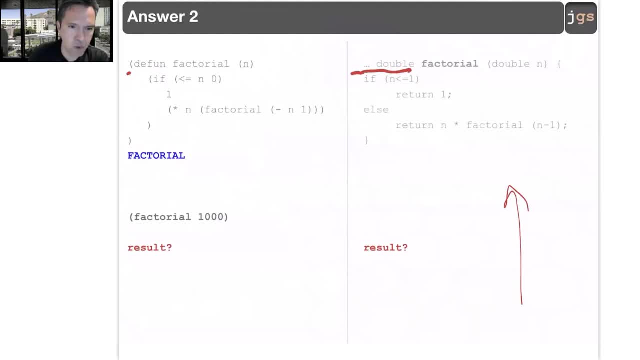 Now the return type is a double. We don't care, We only need to remember that we want to return a number, The name for the function- Now open parenthesis, It's going to close here And inside. definition of a function and the name that I want to use: factorial: The same. 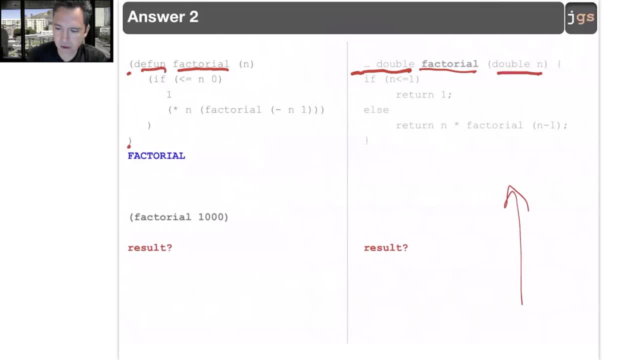 that before One parameter, One parameter, No data types, Inside of the function, the body, this if-else, And I want to return things inside of the if and inside of the else. Good, We have open parenthesis, closing parenthesis and we want this if condition, The condition. 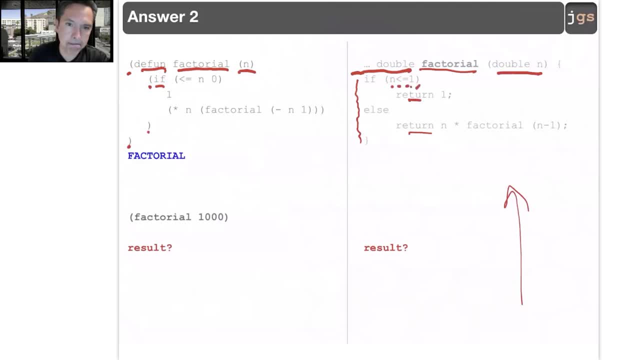 the parameter lower or equal than one. The parameter lower or equal- oops- than one. There you go. Lower or equal than one. The only thing that looks different is that now the operator go first instead of being in the middle. If true, I want to return one. 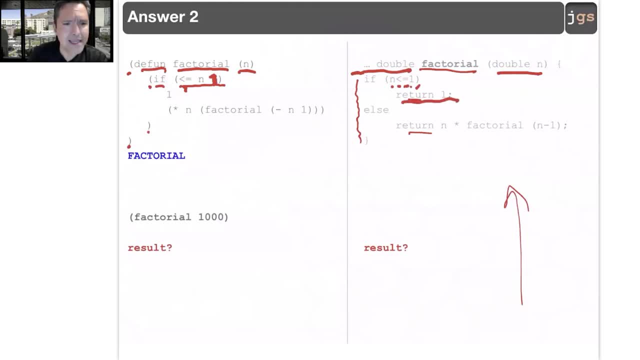 Here. I do not have a return keyword. I do not need a return keyword. The only thing that I need is the value. It's a value. I do not have parenthesis. Therefore, if this condition is true, the only thing that is going to happen is this is the value that the if is going to return. 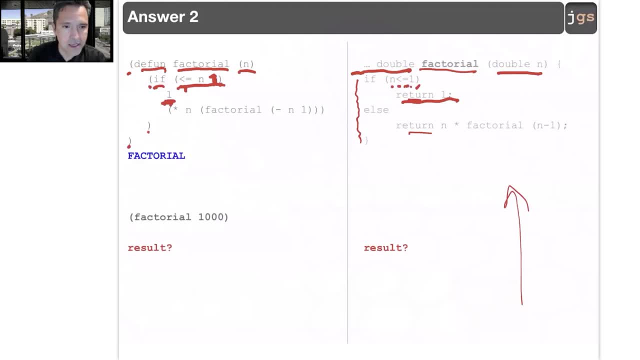 And because the if is the last line, the only line inside of the function, it's also the value that the function is going to return. The function is going to return. So I'm going to return one Notice: no parenthesis, no quotation marks, nothing, Use one. 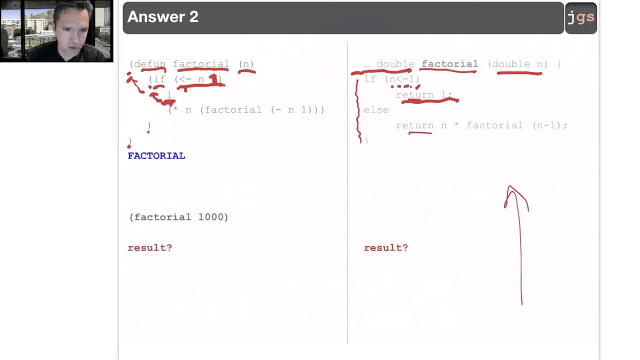 And if you want to put this one here in the previous line, it's completely fine. Remember, the only thing that you need is a white space as a delimiter. That's it. Then the next thing that you want is what happens when the condition is false. 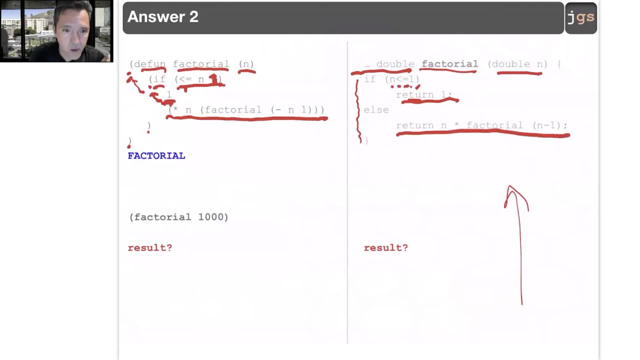 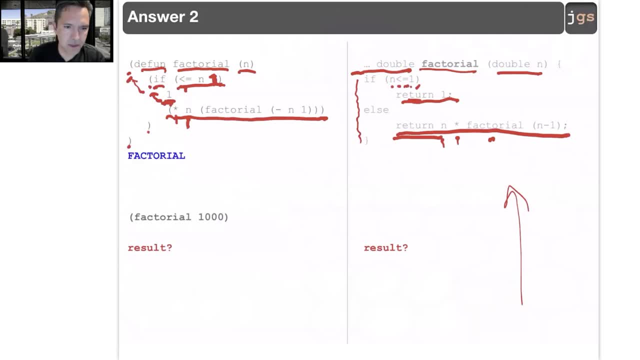 of n, And the second parameter for the multiplication is this one And, as you noticed, open parenthesis, you're going to close- and this is the name of the function that I want to call, And it's exactly the same name as the function that I want the.